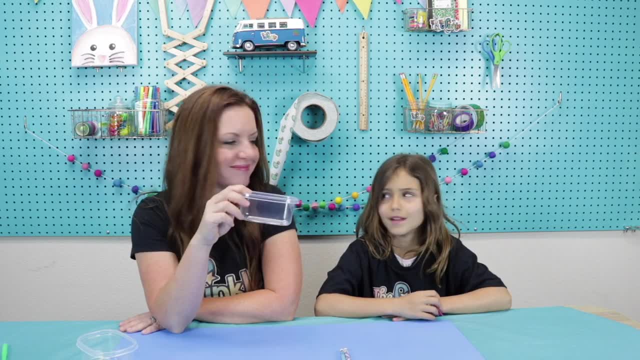 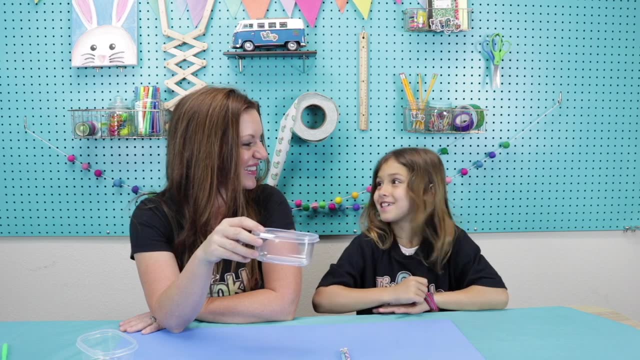 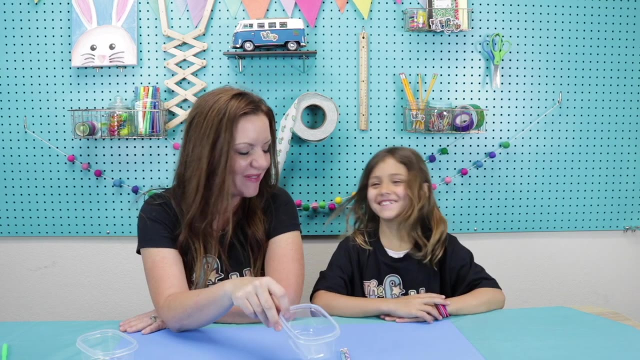 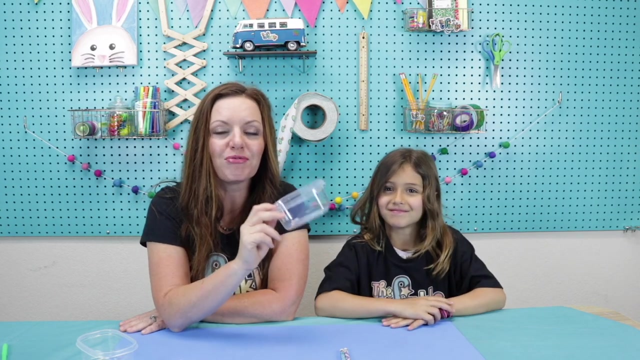 can float in your boat. Do you think a Lego could float in here? Of course, Definitely. What about a stuffed animal? No, I wouldn't take the risk. You wouldn't take the risk. What about our pet dog? No, No, Way too heavy. But maybe a Barbie, Maybe. Maybe- We have to check- Barbies can float. This is a great time to experiment with your boat at home. This project doesn't take a very long. 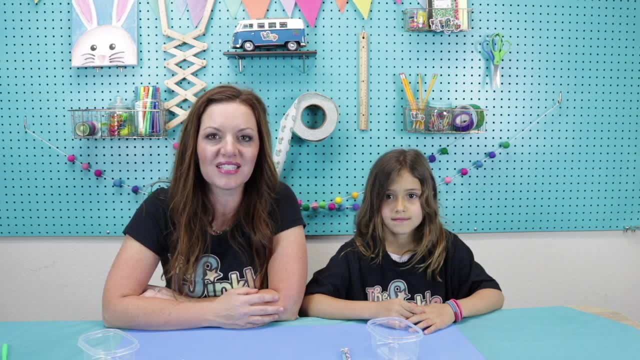 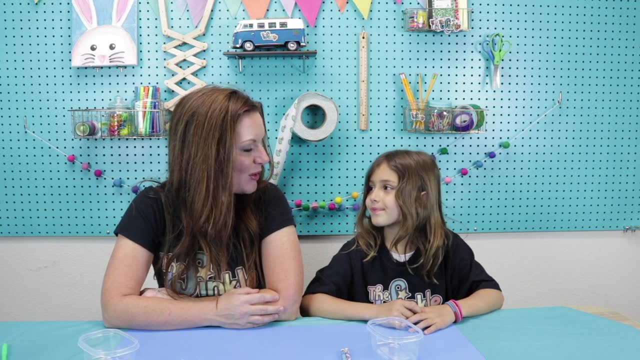 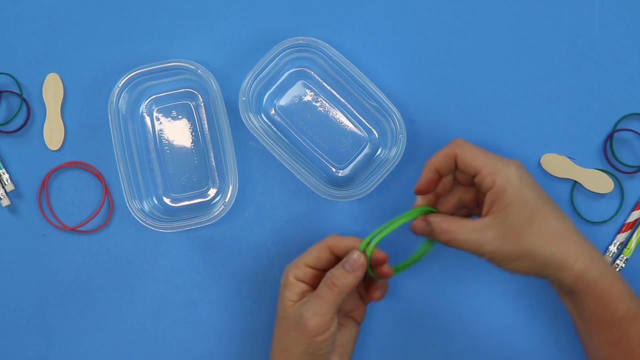 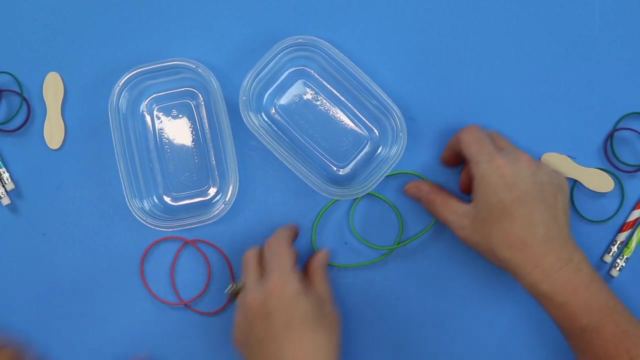 time to make, But after you're done making it, it takes a while to discover what will sink and what will float in your boat. Okay, Okay. So are you ready to get started? Yeah, Let's do it. The first thing to do, Ella, is get your container and your two largest rubber bands. My largest rubber bands are green. Your largest ones are red, So it doesn't matter if it's green or red, or maybe green and red, It's going to work just the same. 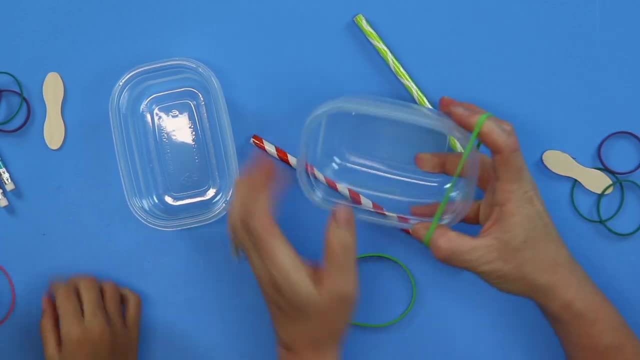 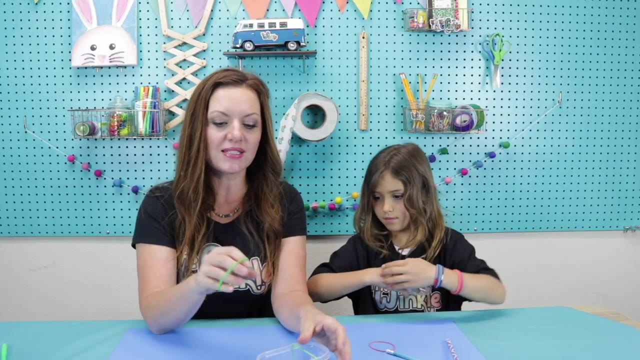 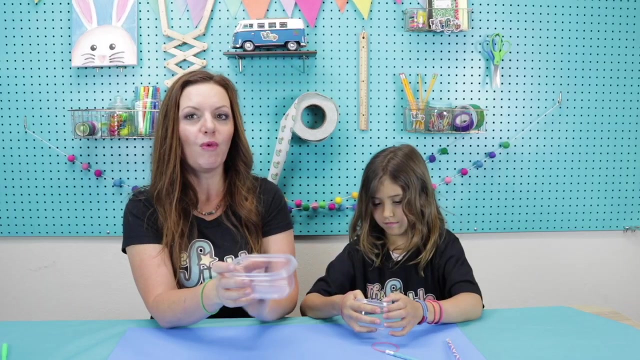 So you're going to, You're going to take your rubber bands and put them at either end of your plastic container And kids, the way to put your rubber band around there. you could do what Ella just did. Ella, you need to show everybody that great trick. What she does is she puts it around. 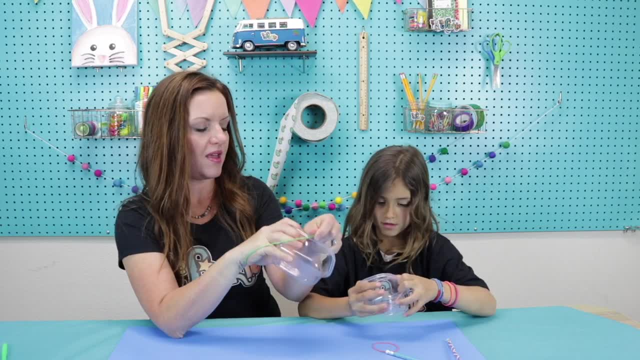 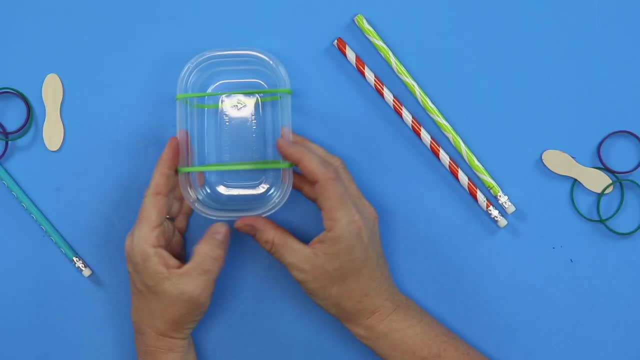 her wrist, holds onto her plastic container and then brings the rubber band over. That's a great trick, But right after it finishes curving like that, that's where you want your rubber bands to be placed. If it's on the curve too much, guess what's going to happen. 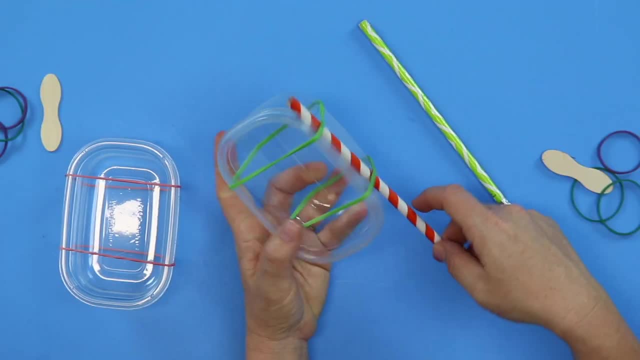 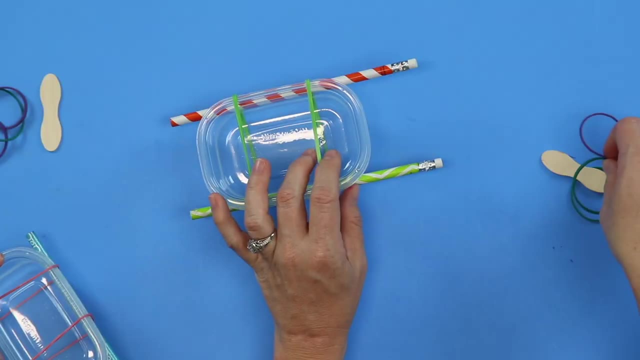 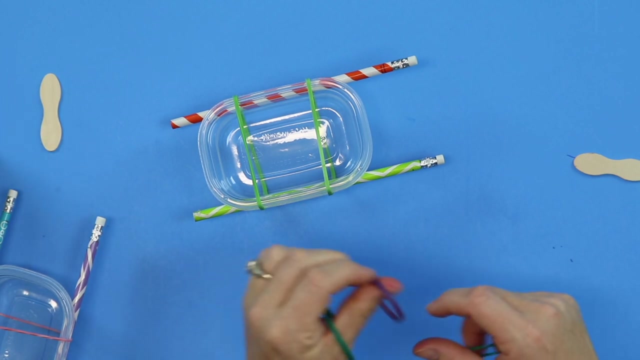 It will just pop off. Pop off. Then you're going to take your pencils and insert them just on the side. Oh, Mm-hmm. Now, this is the only tricky part, so pay close attention. You should have some rubber bands left. The two thickest rubber bands are what we need for this part, So my thickest. 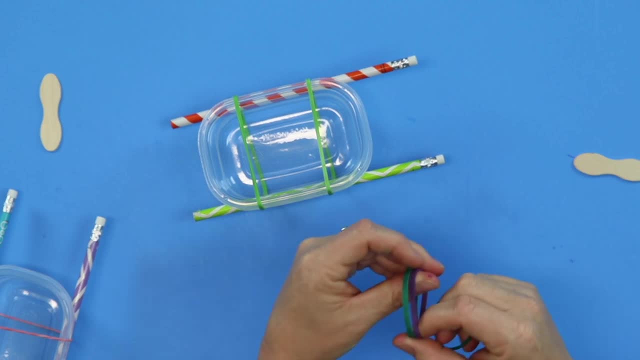 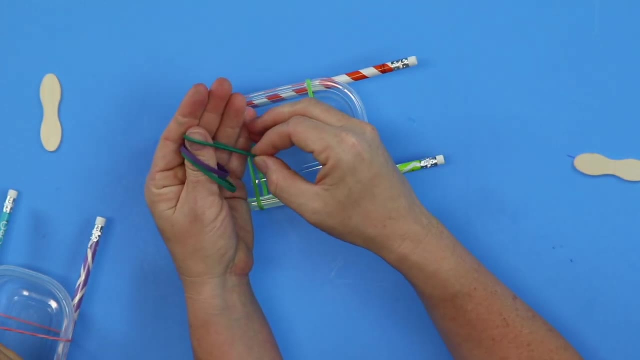 ones are purple and green, Not in any color. One is purple, Two purples, okay. Or you might have two greens And see this one is really thin, so we're going to keep this thin one for later. Do you see the thickness here, guys? 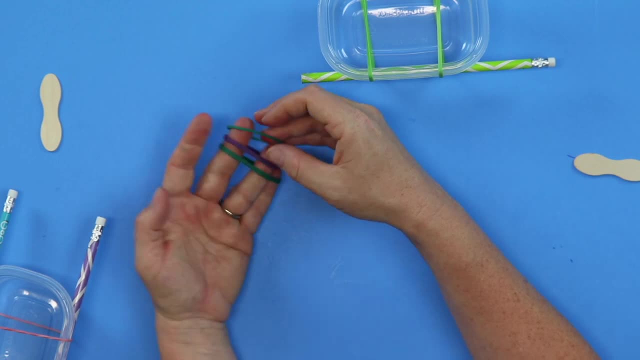 Yeah, Thick means how wide something is, So these two are thick, This one is thin, So the thin one's going to sit out for a little bit and we're going to use these two thicker rubber bands. So we're going to use those fingers. You guys got to use those muscles in your fingers to. 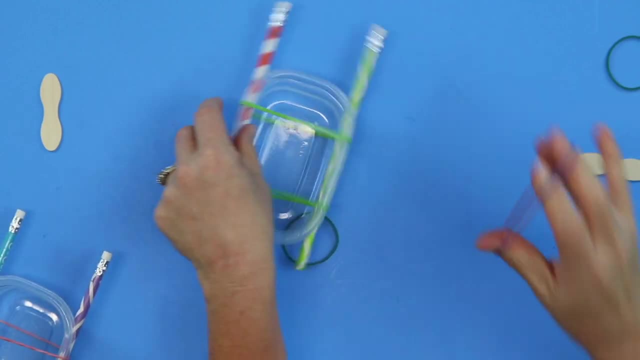 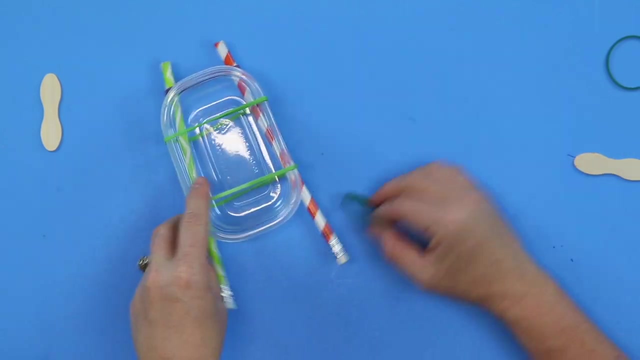 spread your rubber bands, Okay. So you're going to take your rubber band apart- Yes, Yes, You're so strong And you're going to put it around the pencils in the front of your boat. Okay, And then you're going to take your other thick rubber band and put 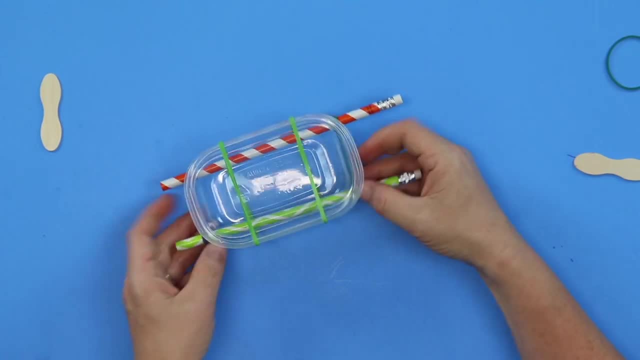 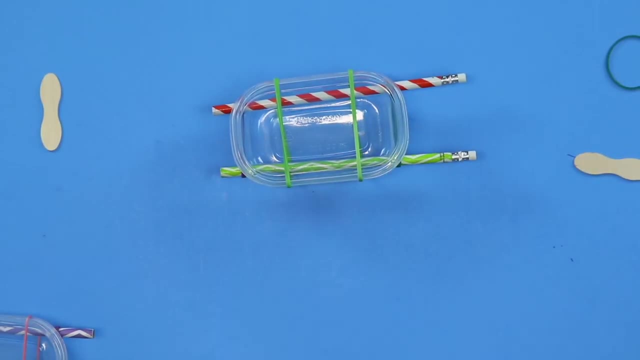 it behind your boat on the other side, And what this is going to do is stabilize your pencils into place. Okay, So how much are your pencils sticking out from the front? We need to scoot them back, Just wiggle them back just a little bit more. Very good, because 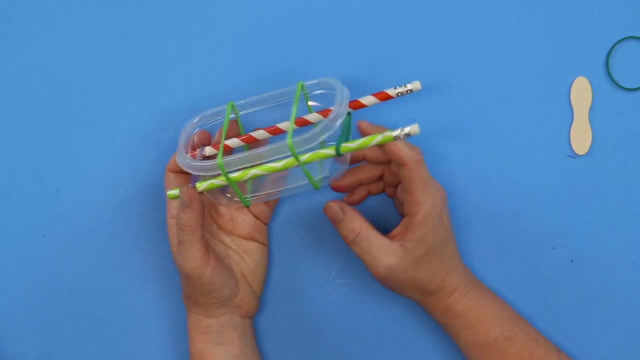 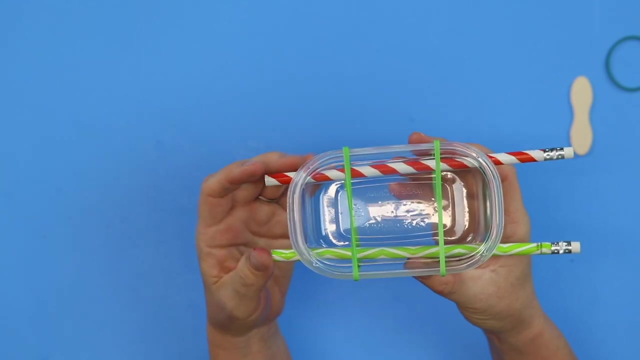 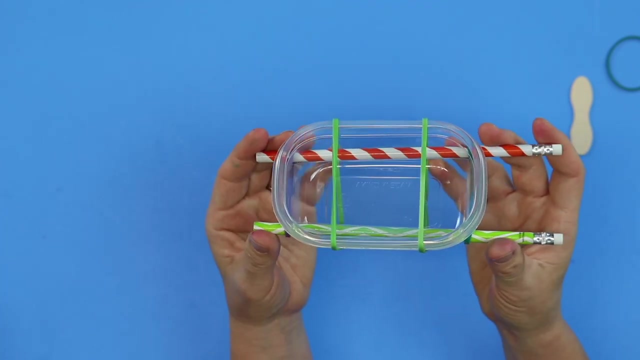 you need enough space back here for your propeller. Good, So we want to make sure that these two thick rubber bands are right up against our plastic container. okay, Like the back ones. Yes, The thick rubber bands are right up against our plastic container because they are holding. 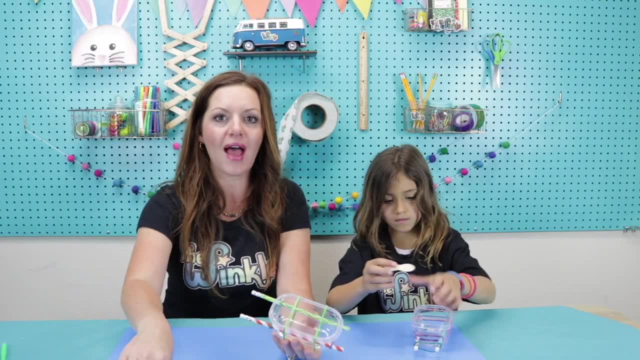 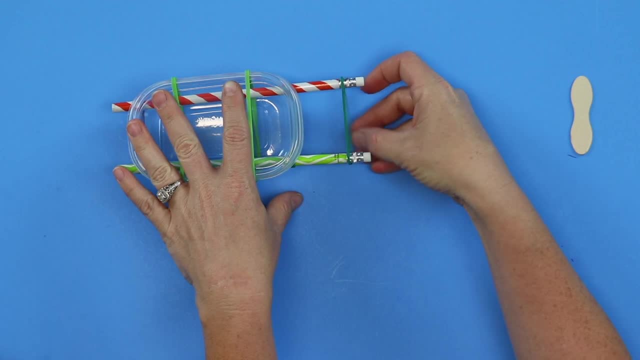 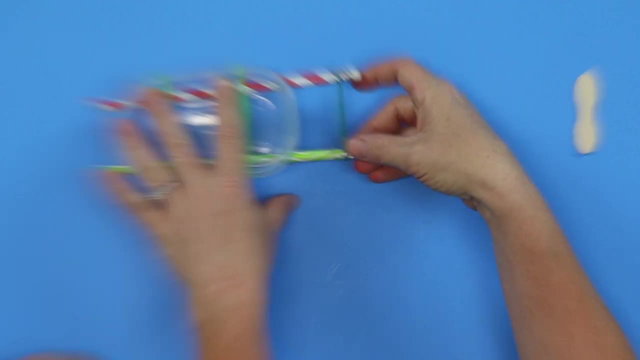 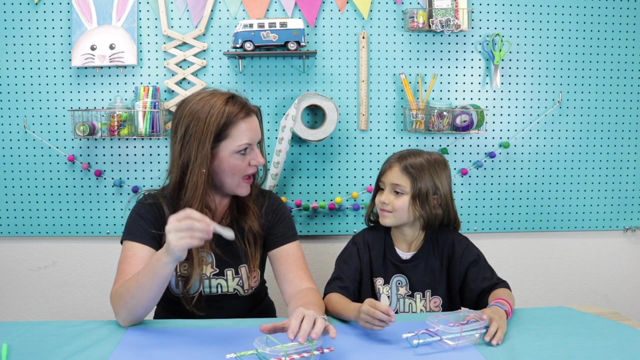 It's going to be great. Okay, so that's this silver part that holds the eraser. Have you ever been on a boat before? Yes, Yes, Of course. And there's a propeller in the back right That goes really fast that. 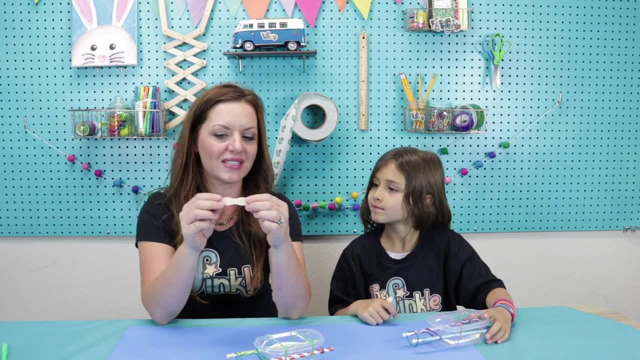 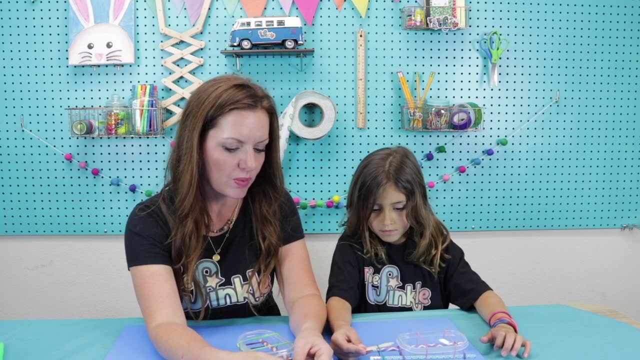 propels. Yes, Yes, propels the boat through the water. So this sample spoon is going to be our propeller, Okay, So the way this works is this sample spoon is going to work as our propeller, just like a propeller on a boat. okay, 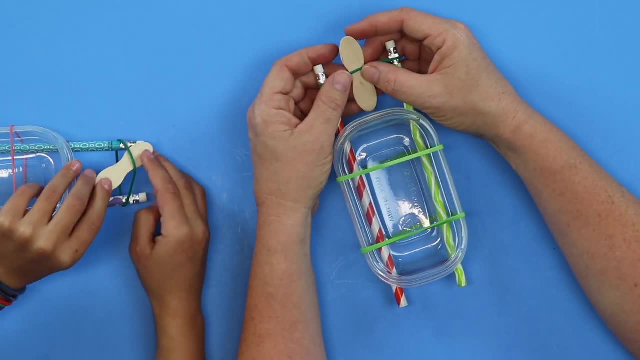 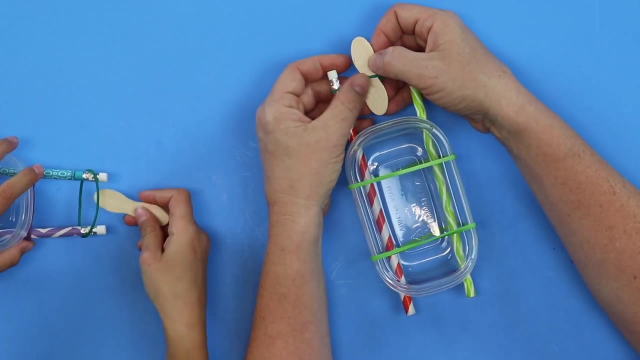 Yes, So we are going to wrap it inside of this rubber band right here at the bottom. Okay, rubber band. see how the middle is in the middle of the rubber band. now let's think about which way this propeller needs to go. ella, we want it to go in the water like this. 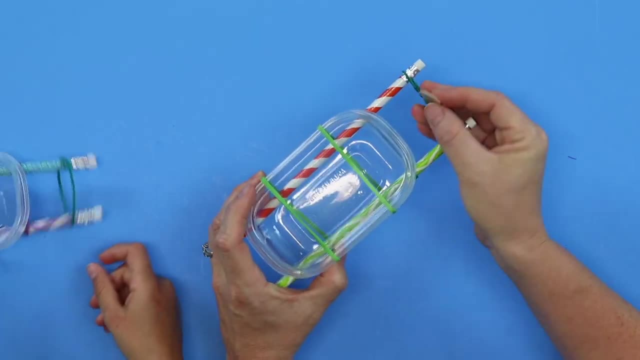 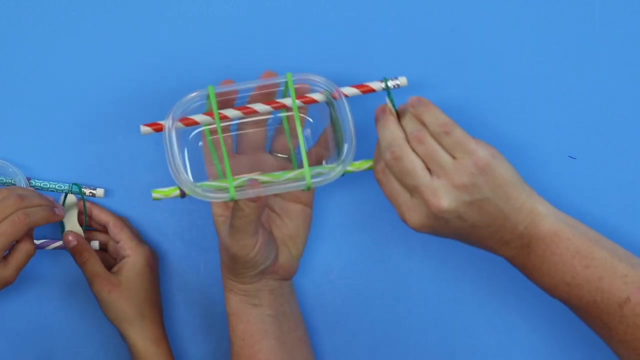 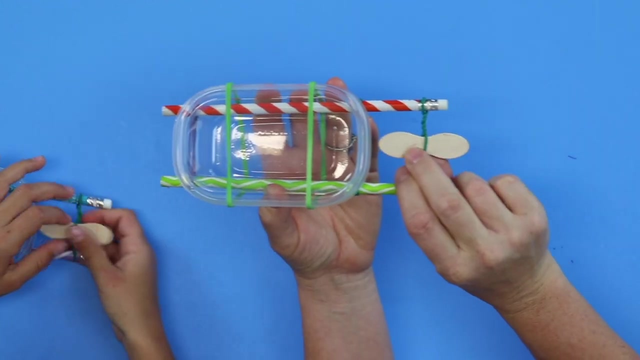 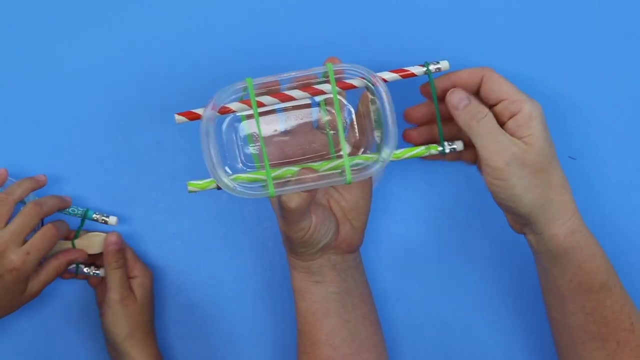 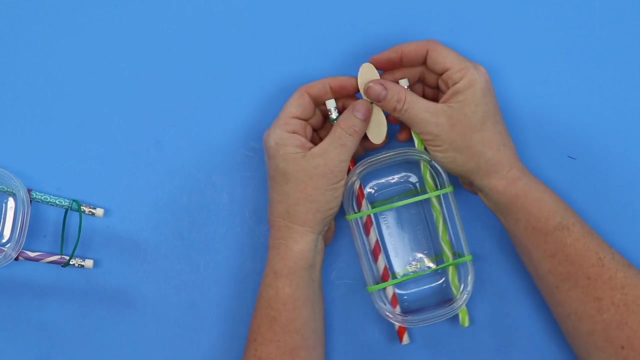 right, flipping towards the boat, because that way the propeller will take the water and push it away from the boat, making it go in the water, right? so we want it to go like this, which means we need to twist it what this way, the other way, so that when we let go, it'll go towards the boat. if you have so, if you have your boat facing you. 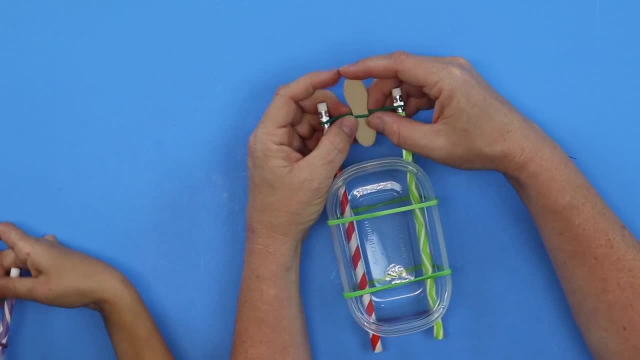 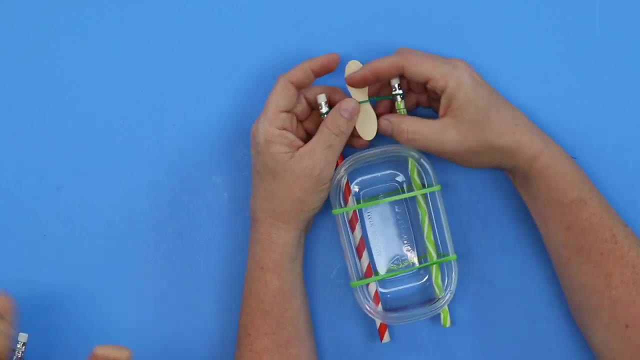 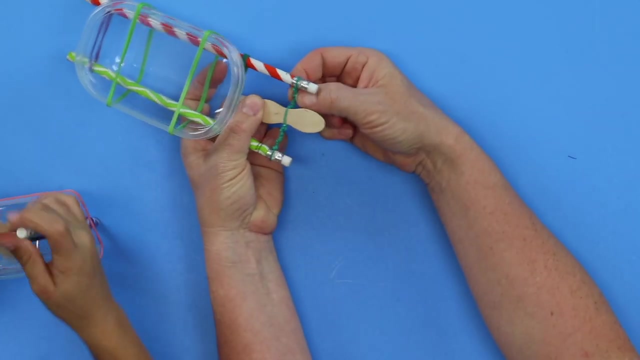 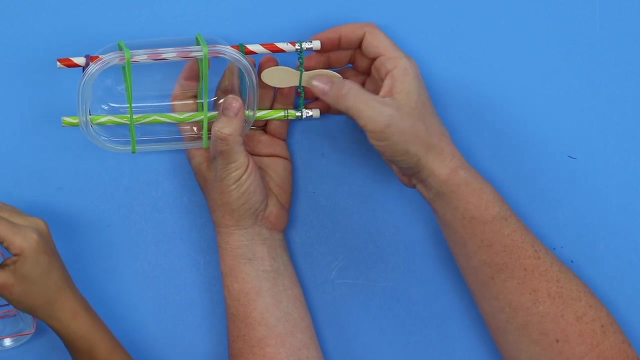 you have your propeller in the middle of that rubber band. you're going to twist that propeller away from you, away from, i know, all of this that's in the rubber band right now. that's called potential energy. can you feel it? can you feel that energy about to just, oh, let go of that propeller and make it? 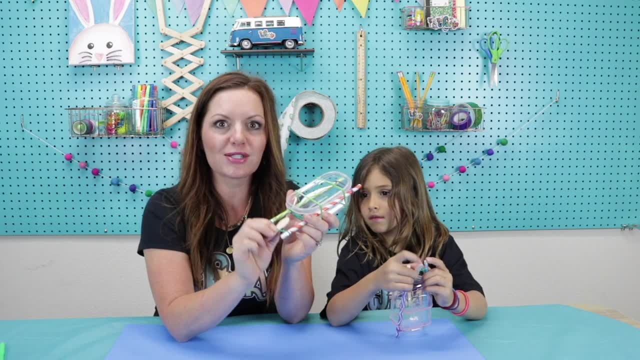 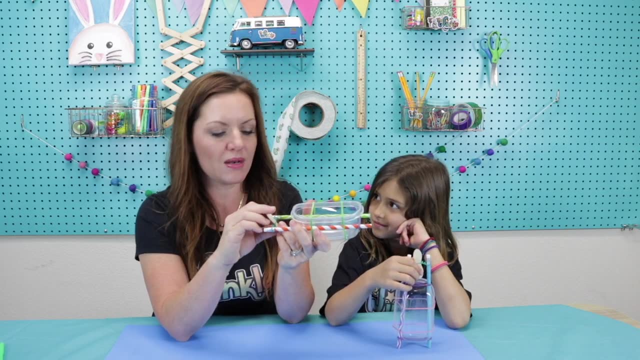 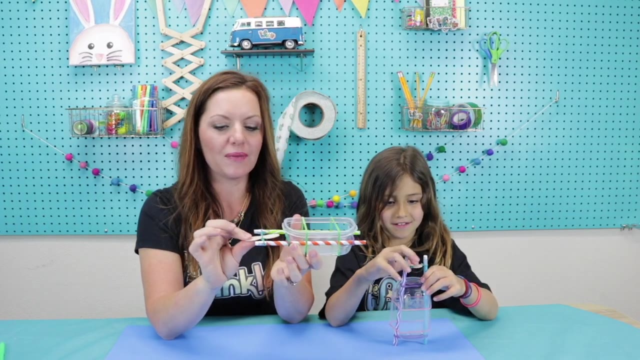 make the boat go. so look at all that potential energy that's stored up in that rubber band just waiting for you to let go of that propeller. it can spin back the other way and make the boat go forward. Isn't that pretty amazing? Yeah, Okay, so we're gonna go try this in our bathtub. Yeah, Alright, we're. 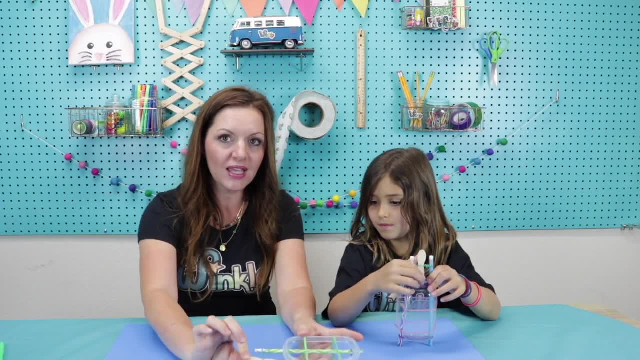 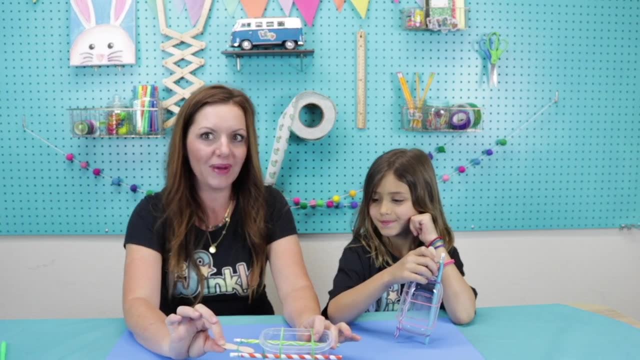 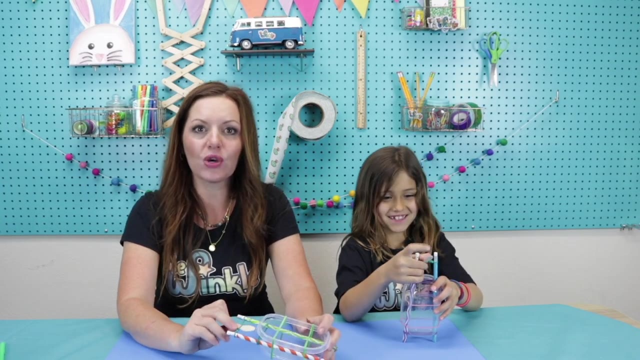 gonna let go of the propeller, but not until the boat is in the water. Okay, so we're gonna put it, our plastic container, in the water, let go of the sample spoon propeller and see how fast our boat goes. And it will go like Yeah, and I think you. 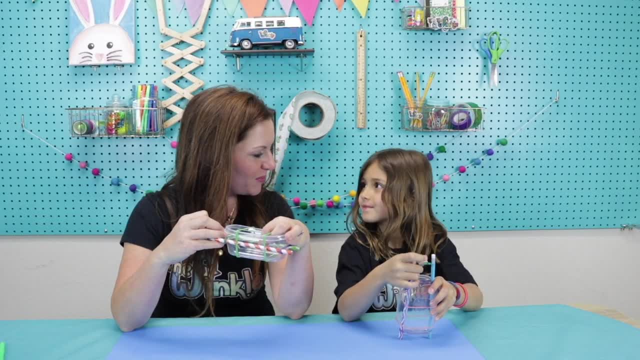 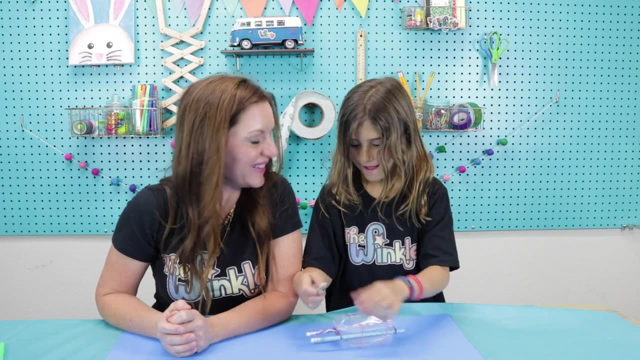 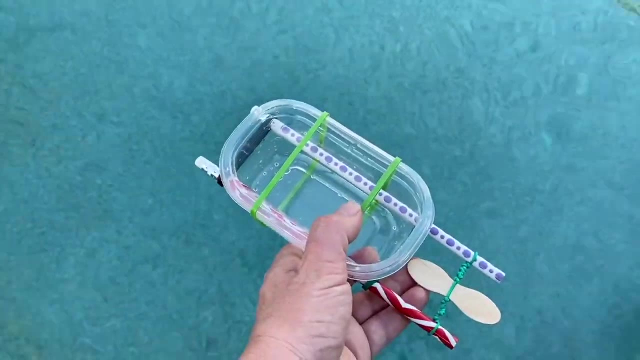 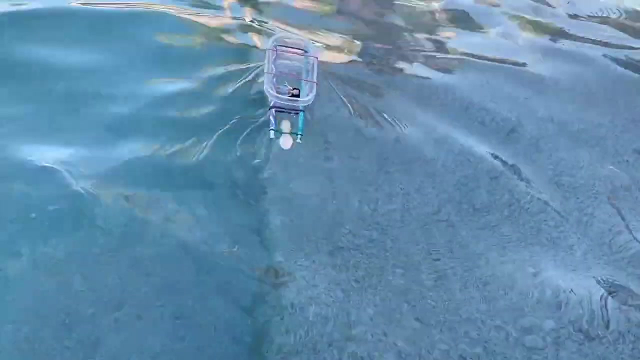 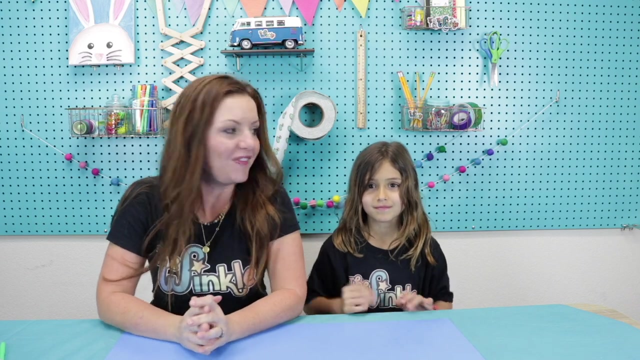 can also try putting something inside of here. Are we gonna try putting in some Legos, Some Lego toys? Oh, that's gonna be awesome. Yeah, Okay, let's go try it out. okay, Okay, That was so fun. Yeah, Elwha, your boat went so great and that was a great idea to put. 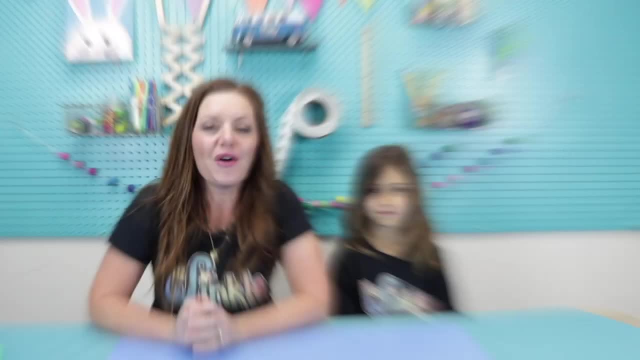 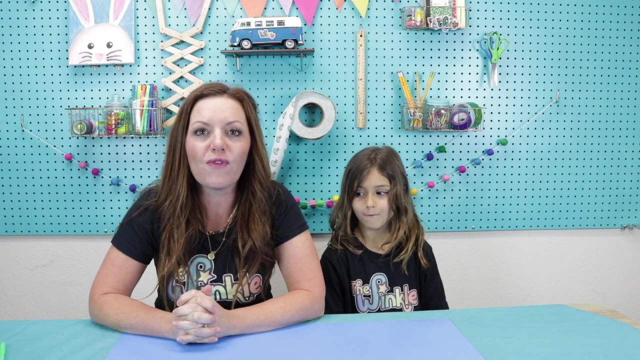 those little Lego girls in there. That was super fun. Yeah, Okay, everyone. we want to see how your boat did. So did you try putting something big in it, Something small? Did it go fast, Did it go slow? We want to see. So have a grown-up, take a picture, or